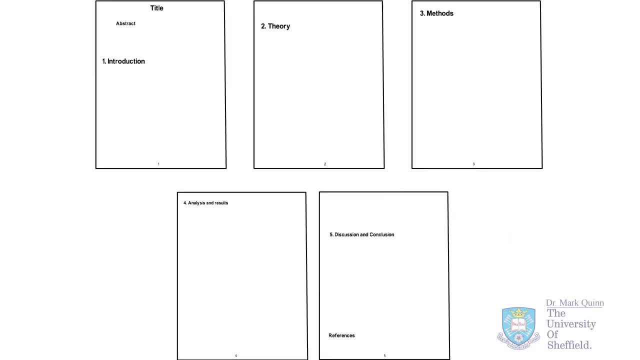 As you can see, a typical short science paper is around four to five pages in length. The lab homework is just the final two sections. The goal here is to practice the two most important sections of a paper. Then at the end of the semester you will have the opportunity to complete the full paper. 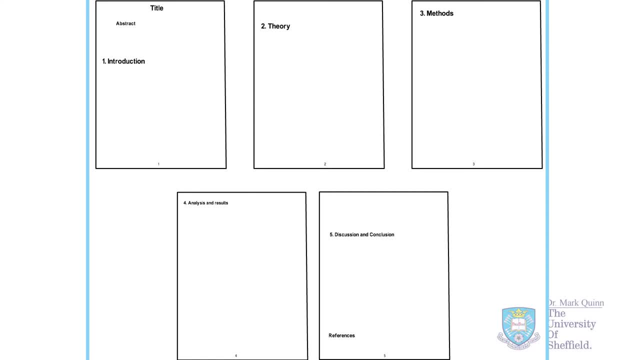 on one of the experiments of your choice and submit this as your final lab report. So you can regard the homework as a mini report on the experimental results of that week, containing just the final two sections, as a brief two-page document. In this demo we will present results from an experiment to measure gravitational acceleration. 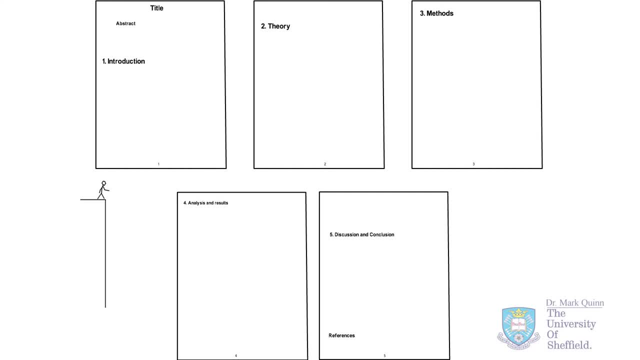 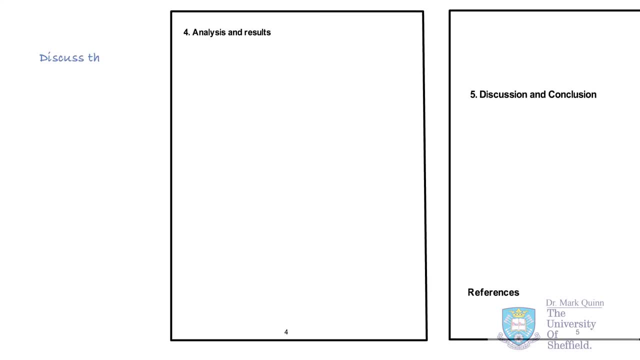 Here the data has been measured by dropping a metal ball and measuring the full time for different heights. Now to get started, let's sketch out the main paragraphs For the results and analysis section. these paragraphs could be discussed: the measured results of the experiment, followed by a graph and a caption to help visualize those results. 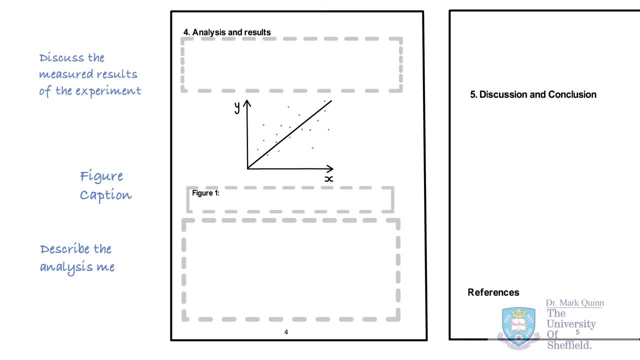 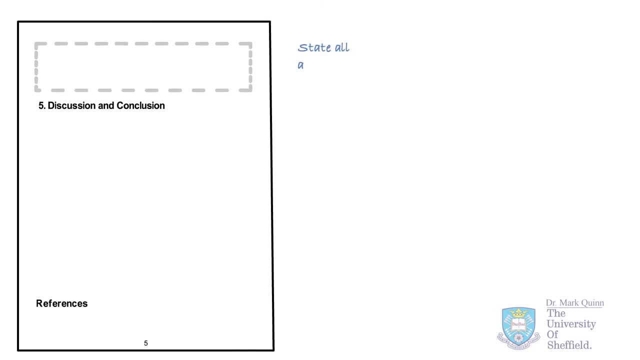 The next paragraph would then be to describe the analysis method, and this will be followed by a paragraph to state all of the analysis results. If there were multiple experiments in this piece of work, you could just repeat this logical structure again. The next section should comprise of paragraphs to summarize and interpret the 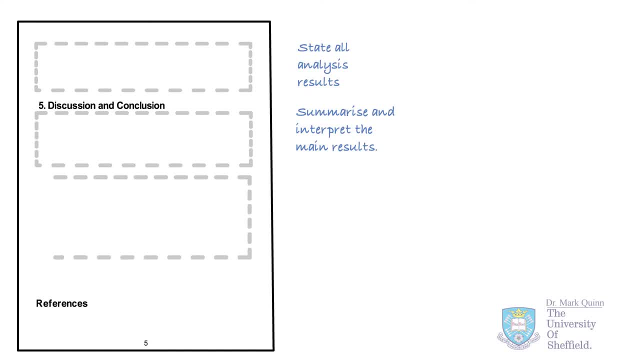 main results. Compare the overall result to the expectation and other published results. You could also describe how your work could be improved in future. And then you finish with a final paragraph summarizing the main conclusions at this point of your work. Notice how each paragraph has a clear and distinct topic. 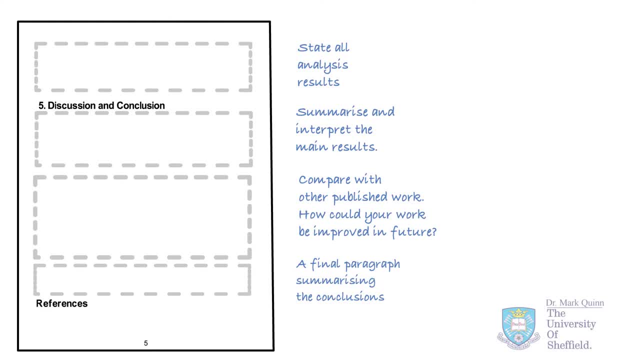 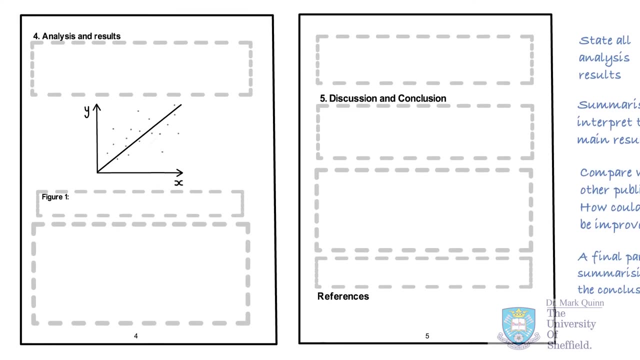 We need to avoid mixing up different topics, as this can be very confusing to read. So let's start filling in these paragraphs and to help both you, the writer, and the reader, it is always useful to start each paragraph with a topic sentence. This tends to be a short initial sentence to set up. 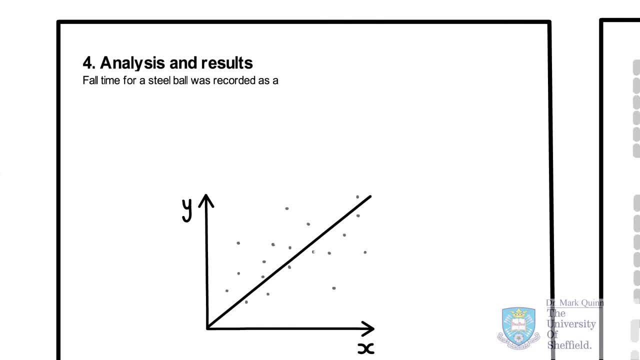 the topic of that paragraph. For example, the first paragraph could begin with: fall time for a steel ball was recorded as a function of fall height. Remember that each sentence sets up the next sentence, So the reader now expects to hear details relating to either the 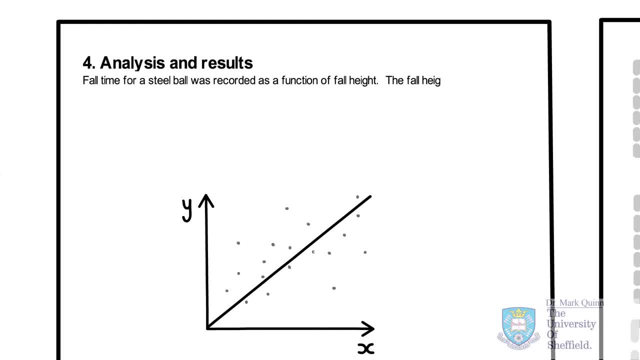 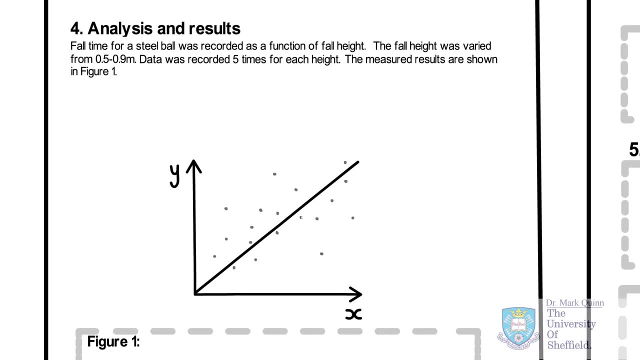 fall time or the fall height. So we will first write: the fall height was varied from 0.5 to 0.9 meters. Next, the reader will start expecting to learn of how many repeat measurements there were. So you can write: data was recorded five times at each height. At this point, let's show the data. 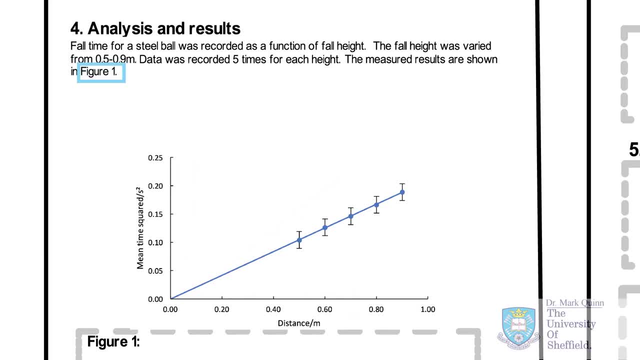 using a graph. To do so, we need to cross-reference the figure in our text, So in this case we can write: the measured results are shown in figure one. Now that the reader knows where to look, we can describe the results. Note, at this point we are only describing the measurements, not the 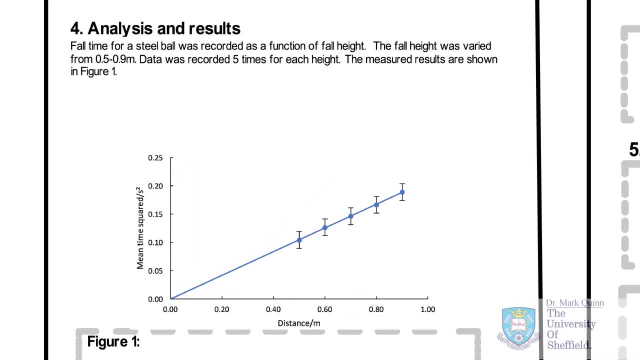 fit line, which is the analysis results. For now we need to tell the reader how the measurements were combined So we can say here the mean of repeat measurements. squared is shown as a function of fall height, So the key word there is the mean. So we're saying that we had repeat measurements. 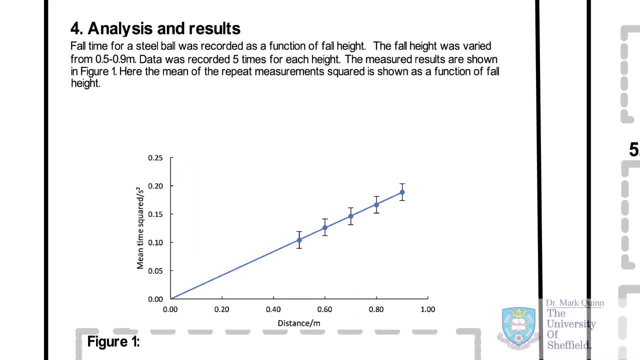 and we combine them as an average or mean to present here. Ensure that you clearly describe how the error bars were then calculated. For example, the error bars represent the error on the mean fall time. Then you can provide extra detail to ensure that there's no ambiguity about the error bars. So we can say: note that the error 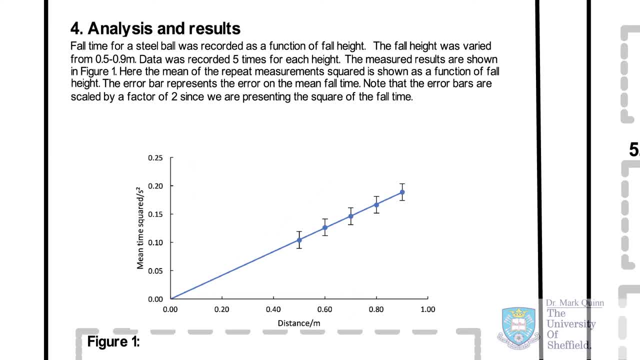 bars are scaled by a factor of two, since we are presenting the square of the fall time. So this is basic error propagation. If you square a result, you double the error. Next we could describe the data. For example, we could write that the measured data has no outliers. 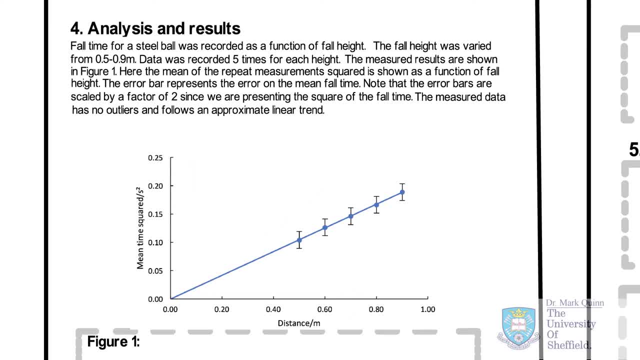 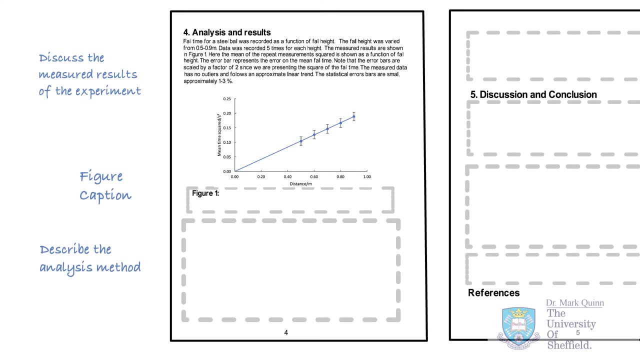 And it follows an approximate linear trend. We can also describe the overall statistical errors by writing. the statistical error bars are small, approximately one to three percent, So we have now provided a summary of the measured data and this now exists as a separate paragraph before we get into the details of analysis and other processes that we can do, Before we get to the 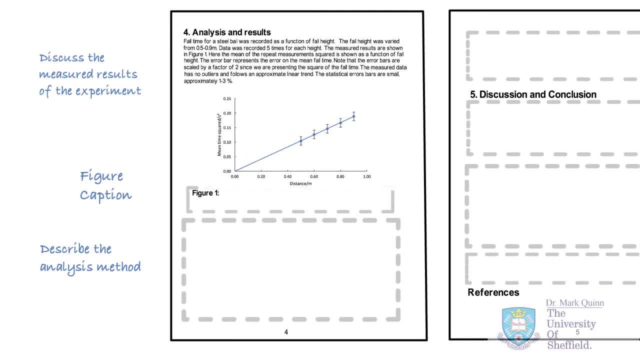 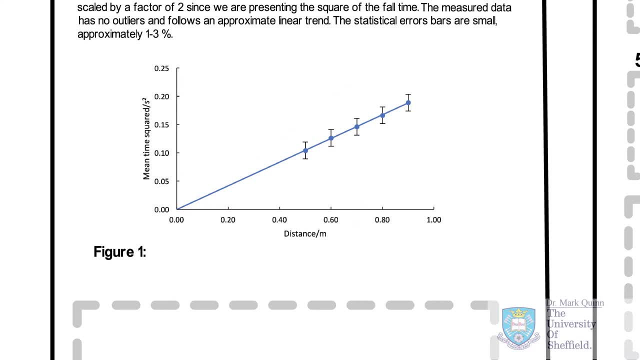 analysis. we should include a caption on the figure because, remember, many people will briefly look at the figure before they read the main body of the table. So we can say: note that the error bars are scaled by a factor of two, since we have no ambiguity about the error bars. So the caption serves as a 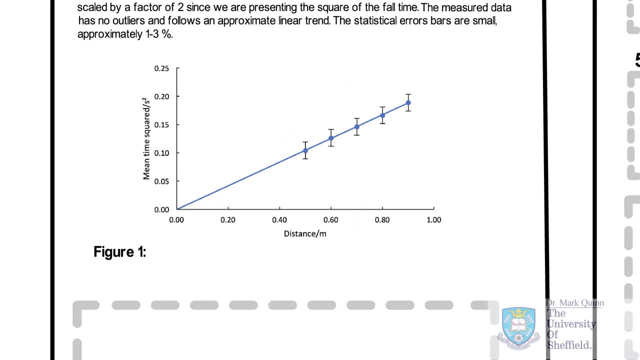 little concise summary of what's depicted in the graph. We always start our captions with a brief summary sentence to state the source of the data. So in this case we can write experimental measures of free fall for a steel ball. Next, after the summary sentence, we can provide more detail. 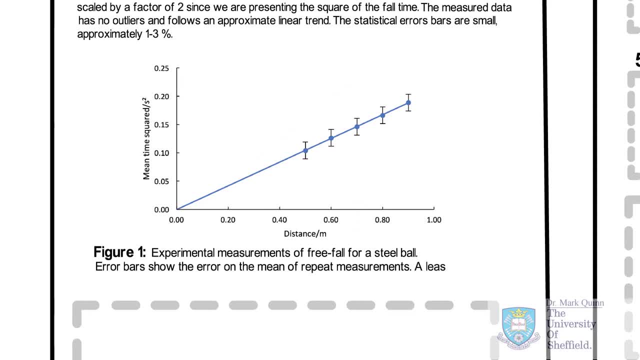 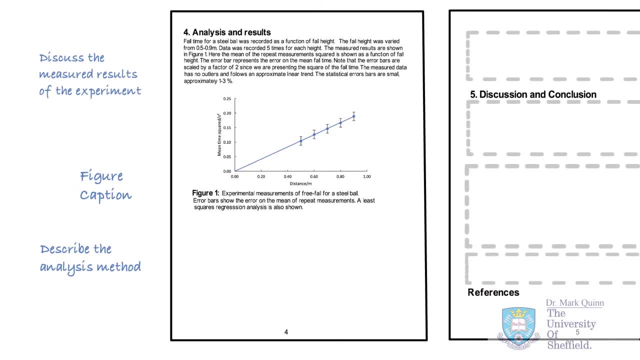 on what's depicted in the graph. Remember, we typically don't state any analysis results in the figure captions. The first step of the analysis paragraph is to state motivation. What is it that we want to determine? Again, as with every paragraph, we start with a topic. 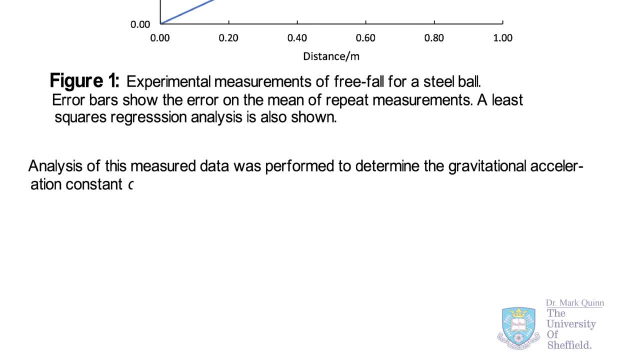 sentence that's short and concise. Here we can say that analysis of the measured data was performed to determine the gravitational acceleration constant g. So now the reader expects to learn about what the analysis was and how we determine the value for g using this analysis. To begin, we 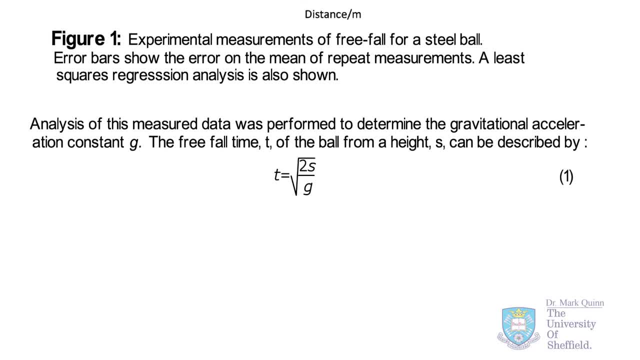 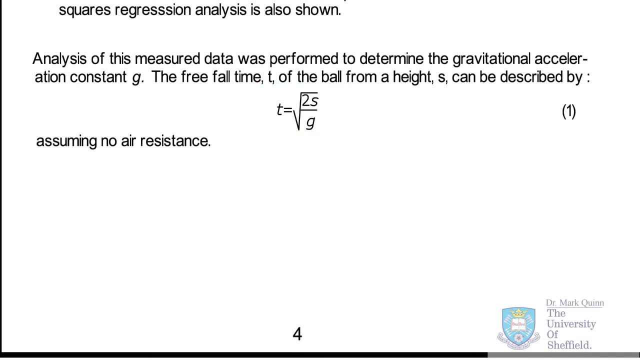 can state the theoretical model that we're using in our analysis and notice that the equation is given its own line, It's centered on its own line and on the right hand side, towards the margin, there is an equation number and we can use this equation number later in the text. 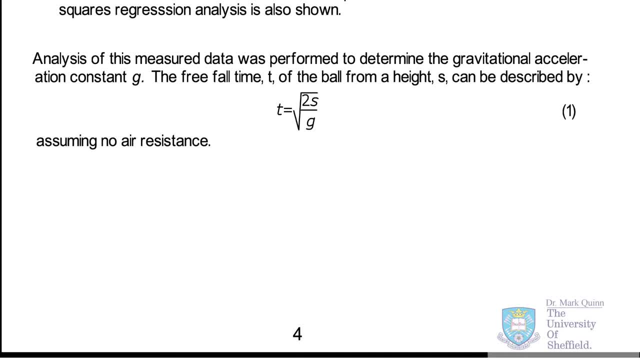 to cross-reference this equation. If we were writing a full scientific paper then more than likely these theoretical equations would have been presented in the earlier section called theory. So this is the theoretical model. Next, we should make clear to the reader how we analyze the. 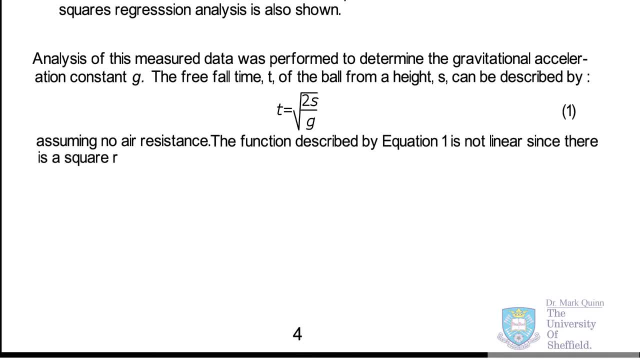 data. First we can state the obvious: that the function depicted in equation one is not linear, and while we could have performed a non-linear analysis, here we are using a very simple linear analysis. So in this case we're going to tell the reader that we linearized our data so that 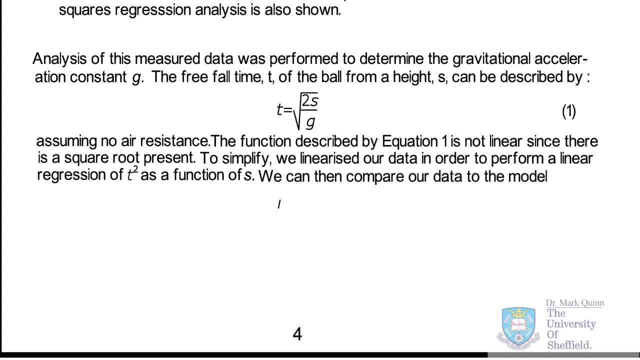 we could model equation one as a linear function of t squared as a function of s- the distance. Next, we should tell the reader what analysis algorithm we used to carry out this process. Here we used what's called the least squares method. Now, this method does not include the 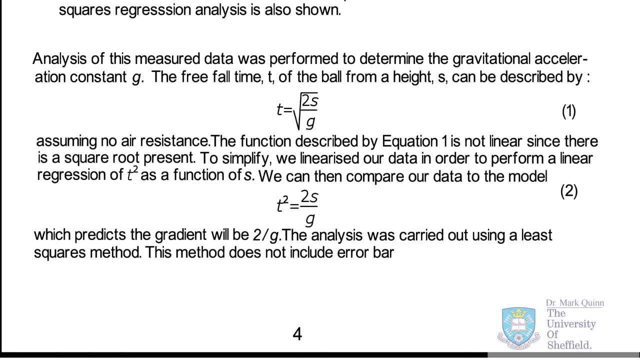 error bars in its calculation, so we should state that explicitly. If we wanted to use the error bars in our analysis method, we would have to use what's called a chi-squared regression In our case, because the error bars are relatively the same or relatively uniform. 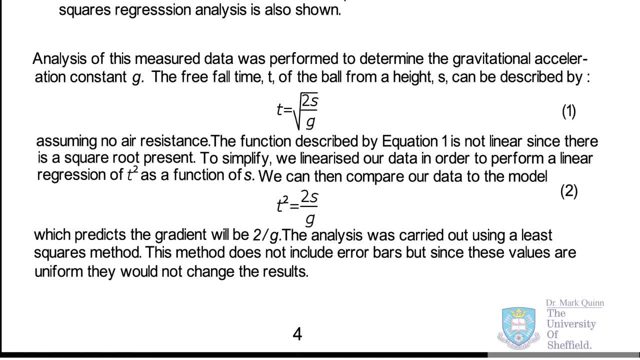 they will effectively cancel out in the analysis. but in cases where the error bars are varying quite a lot, then you should use this weighted chi-squared method. A key aim of this analysis paragraph is to clearly define and describe the analysis method, because the next paragraph we're going to state the analysis results. so we want to convince the reader. 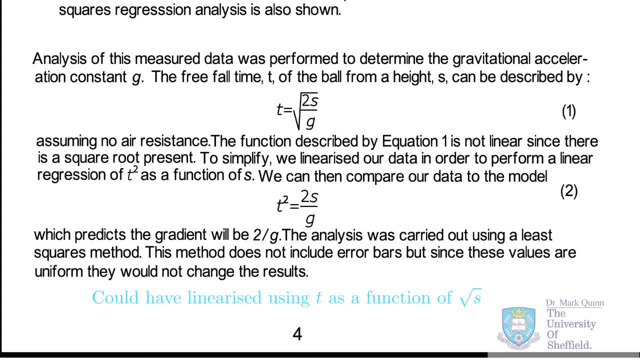 that our analysis method is valid. So if this paragraph is confusing or if it's missing details, you may lose the reader at this point. so even when you show them your analysis results, they may have already given up on you as a scientist, because your analysis method is full of holes. 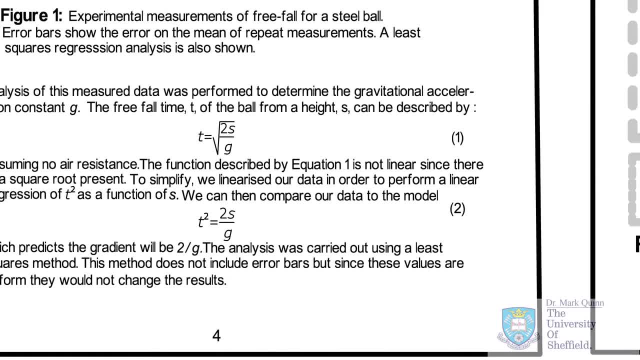 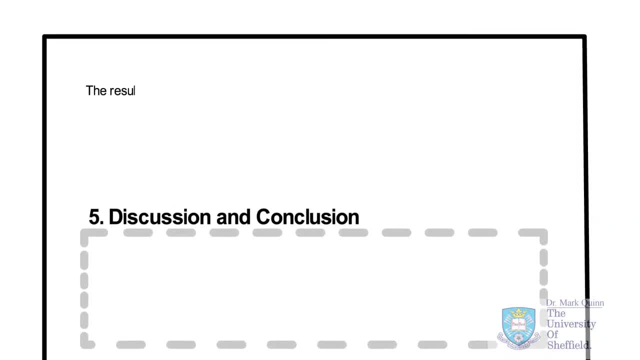 or lacks detail. Now this next paragraph is potentially the most important paragraph of a scientific paper. This is where we get to state our analysis results, the key results of our study. We do not offer our interpretation of the results here, remember that will come later. So 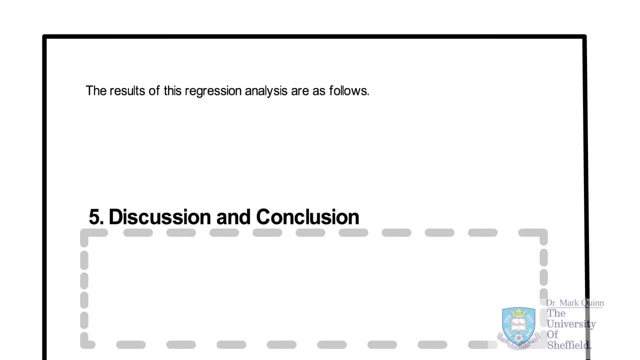 let's start with a topic sentence, again to provide the reader with an impression of what this paragraph we'll discuss. so here we can write: the results of this regression analysis are as follows. we then state the results of the regression analysis, which are the slope and the intercept. 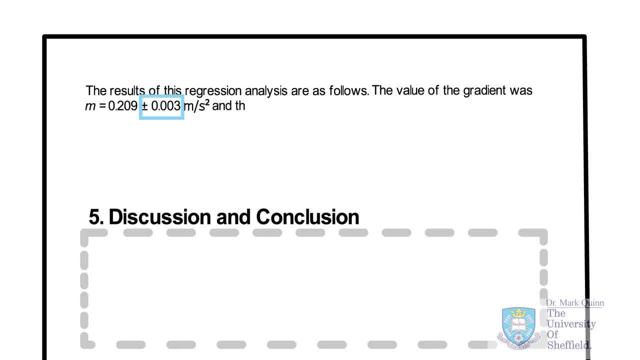 parameters together with their statistical errors. note here that we've rounded the error to one significant figure. in both cases this gives us three decimal places of precision. we then write the result value, the same number of decimal places as the error values. the next analysis result is the goodness of fit, or the correlation coefficient, or squared for a perfect linear fit to the data we. 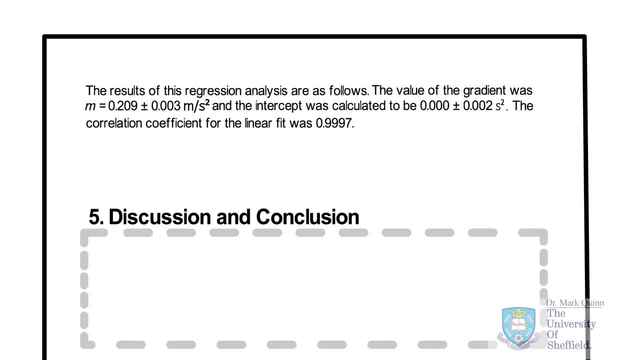 expect this to be one, or very, very close to one. now we can use the regression results to calculate another result. in this case, we are calculating a value of g, the gravitational acceleration. in most experiments that you do typically, your regression analysis will give you some fit parameter, like 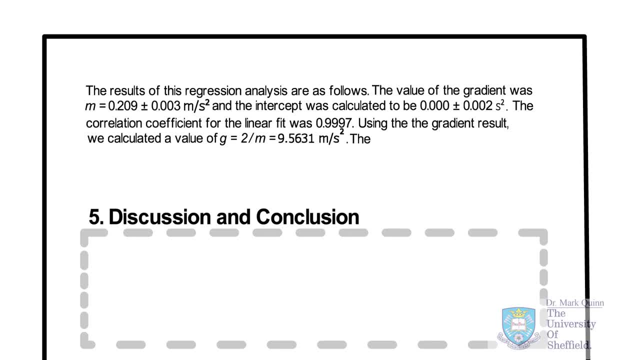 gradient, and then you will use that fit parameter to determine a physical property of the experiment that you're trying to measure. we then have to ensure that we describe to the reader how we determined the statistical error on this physical property, and here it's quite simple, since we're only using the value of the 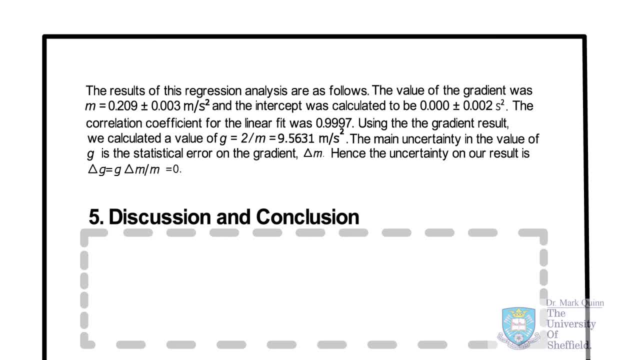 gradient. it is only the error on the gradient, or in this case the relative error on the gradient, that provides us the relative error on the physical constant we are determining, called g. once we've done that, we state the final value of our result again, together with the statistical. 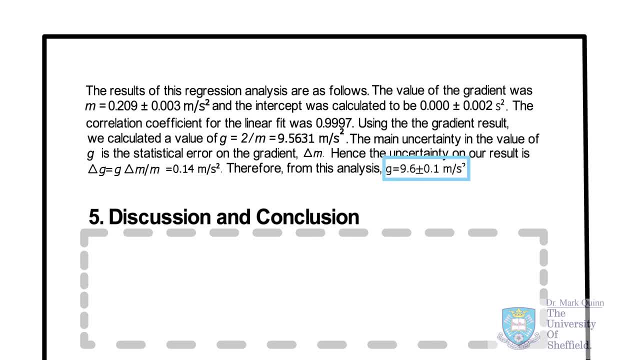 error, which is again rounded to one significant figure. in both cases, this gives us three decimal places of precision and we round the result value, 9.6, to one decimal place of precision. this is now the end of the results section and there won't be any more results introduced for the rest of. 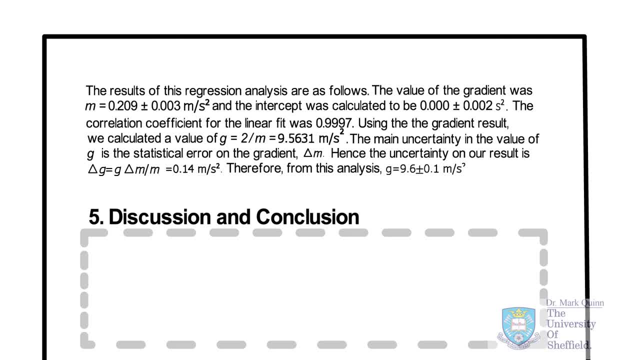 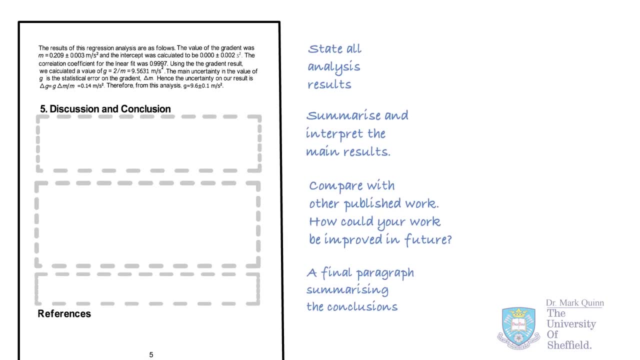 the paper. the main aim of the discussion section is to turn these results and the data into knowledge. this is where you get to sit back, interpret what the results mean and then to put these results in some broader context in the first paragraph of the discussion section we're going to 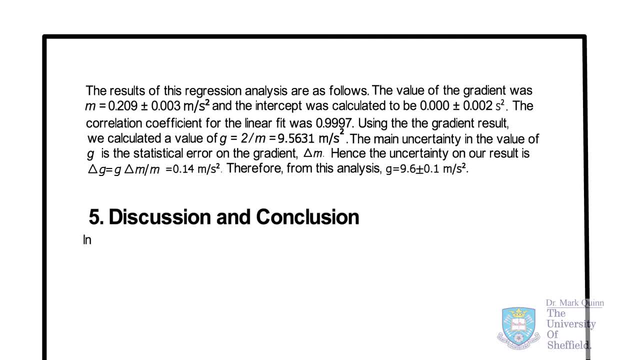 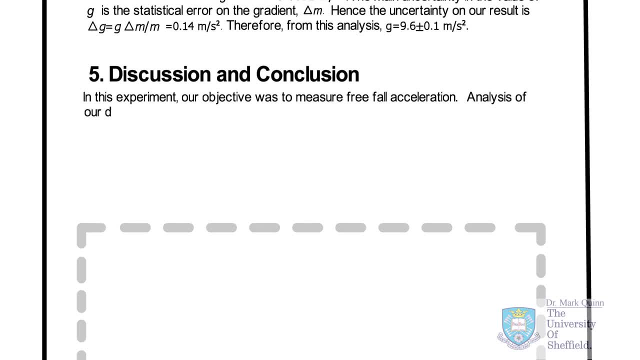 then, to put these results in some broader context, in the first paragraph of the discussion, you should aim to remind the reader of your original research question here. this was to measure the free fall acceleration. next, you should provide a summary of your results and interpret the results in order to 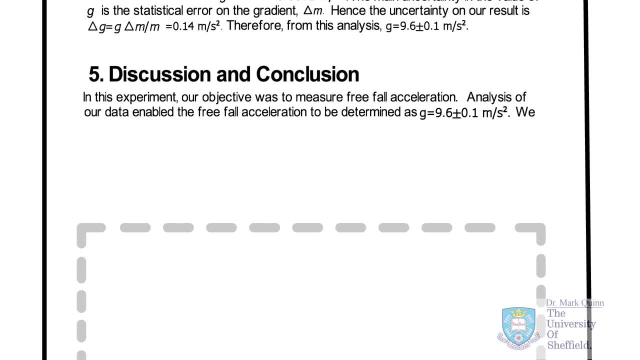 answer this research question. a key part of this interpretation is to bring attention to the uncertainties in your analysis results. here we can bring attention to, firstly, the statistical error. from our regression analysis we can attempt to describe possible systematic errors and again we can try to draw down the data to the point where what the error was, this was performed or we can try to work through it, we can try to describe the. there are often some errors in the interpretation. we can see that the error in the data is not the psychological error, but the incident error is the error in the data. so this is not the study error, the achievement error, or we can try to caught up with the. 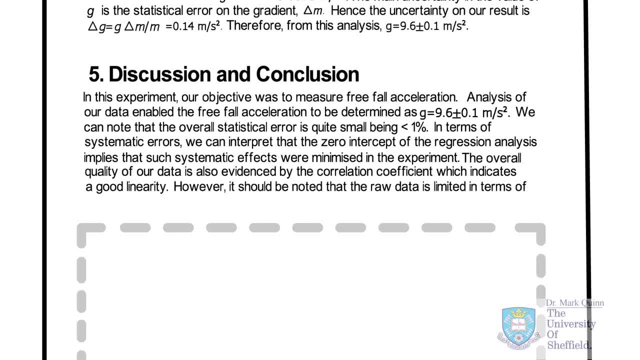 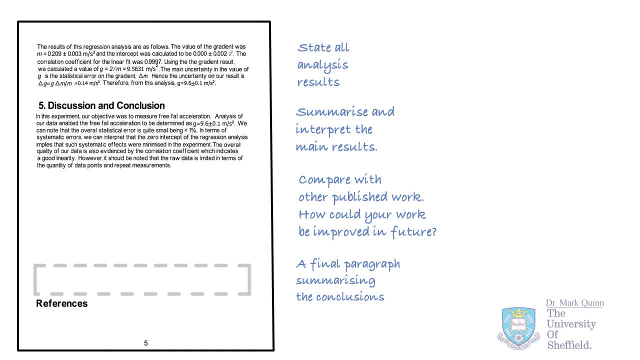 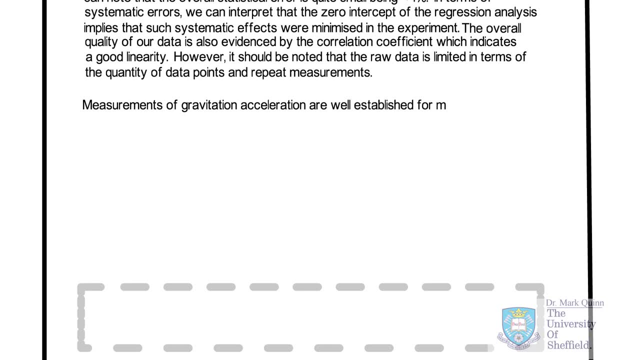 again, we can use our regression analysis results to do so. Now that we've interpreted and summarized our main results, we should attempt to put our results in some broader context. A typical way to do so is to look at the published research literature on this topic. How do our results compare with? 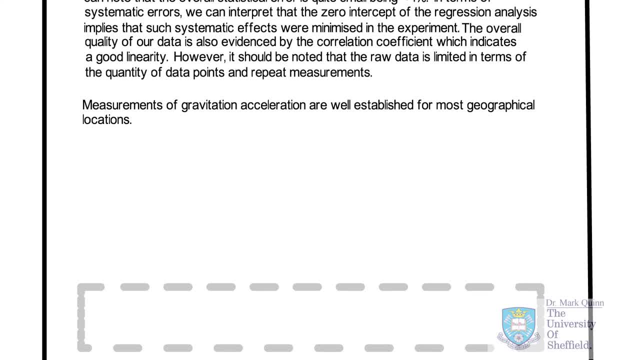 what we'd expect from the published literature. Are our results completely new and novel, or do they support previous work? If you cannot find any published results that are directly relevant to your main results, then you can still aim to put your results in some broader context. For example, what is the?